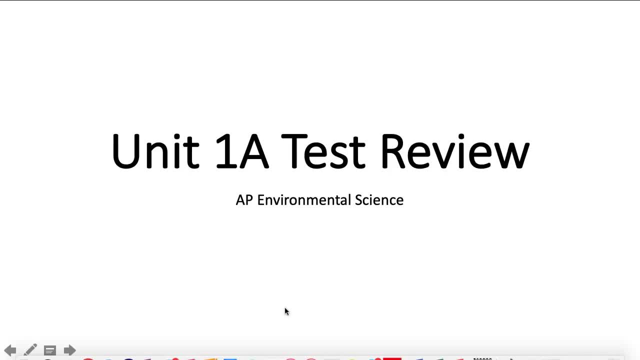 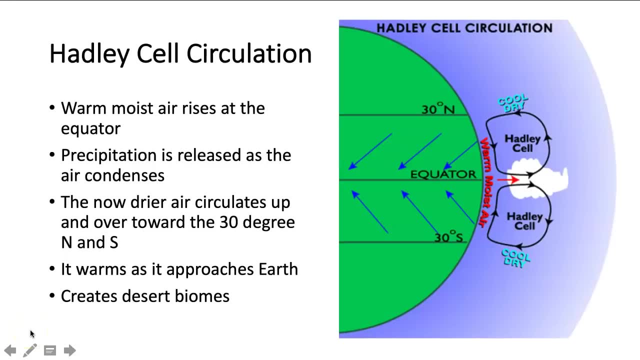 10-15 minute warnings to make sure you are on pace to get ready to finish up on time Once the bell rings. test gets submitted and we're done Alright. so let's start with reviewing a little bit about biomes and the different types of air. 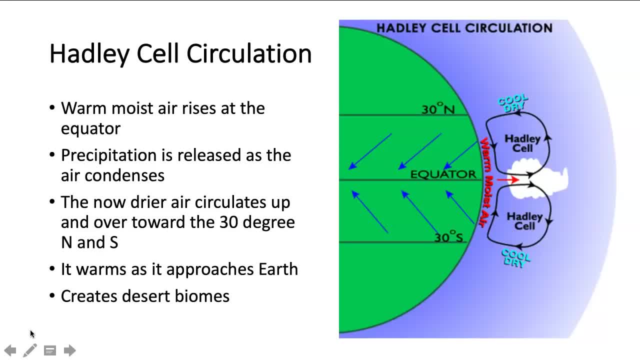 circulation and climate issues that you will need to know about. that will influence where biomes are located- One of the first things we went over in class, and you should have a picture of this drawn in your notes as well, and I'd highly recommend going back over your notes in. 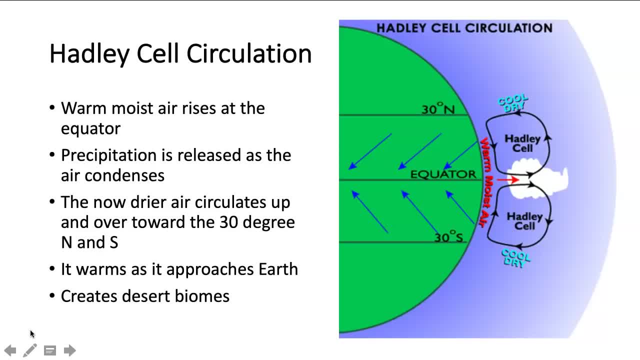 addition to this video, Hadley cell circulation is something you will need to know. If you look at the picture that is on the right, you guys will need to know that Hadley cell circulation, as you can see, is going to begin at the equator, so that's going to be at your zero degree. 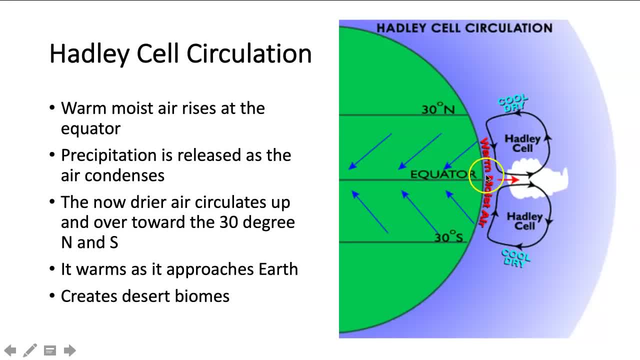 latitude mark, You are going to have air circulate up and over, as you can see in the Hadley cell picture. Notice that the warm, moist air that is going up into the atmosphere is cooling and drying down because it's releasing a lot of its precipitation or moisture. All of that kind of gets. 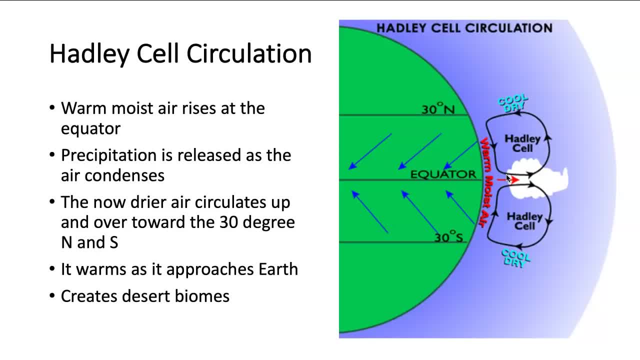 over the rainforests around the equator, hence why there's a lot of rainforest there. but as that cooler and drier air circulates up and over towards the 30 degree north and 30 degrees south mark, you can see that it is going to be. 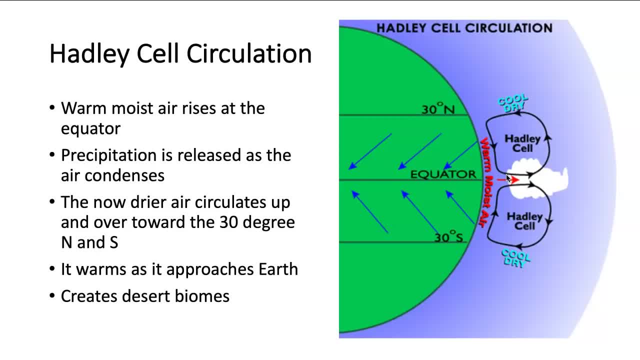 drying out and sinking, but as it sinks it's also going to warm back up as it approaches the earth. So consequently, around those 30 degree north and south marks, we tend to see a lot of deserts and, in fact, if you were to go, look at a. 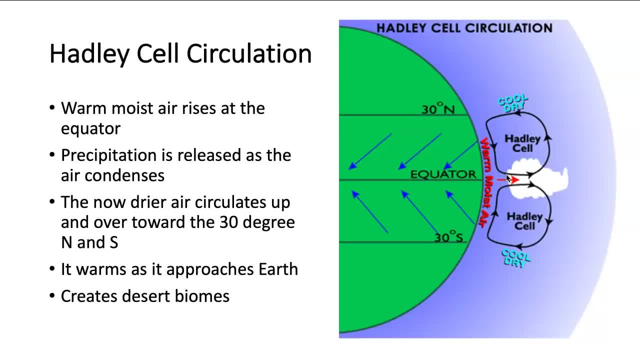 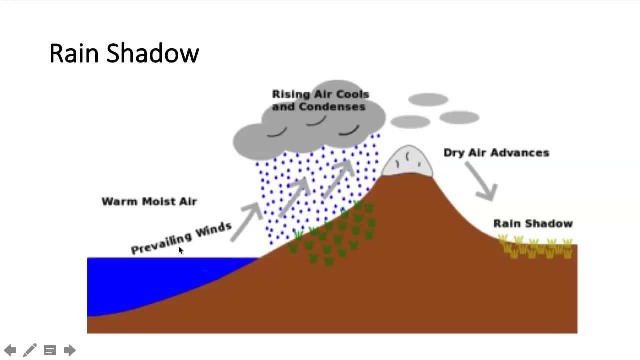 map and find where the Sahara Desert is in Africa. you would see that it lines up really close to that 30 degree north mark. Okay, another environmental aspect of biomes you should be familiar with is the rain shadow, which it seemed like a lot of you had some trouble with this. 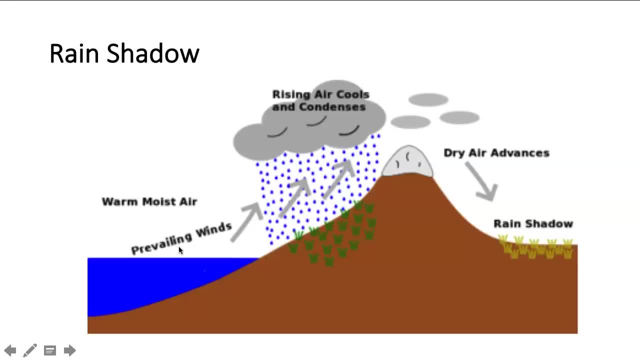 question on the assignment that we did in class. So what you should be aware of is that rain shadows normally occur when you have warm, moist air coming off of something that's not really wet. So if you have a rain shadow that's not really wet, you're going to see some kind of coastal area heading towards mountains. 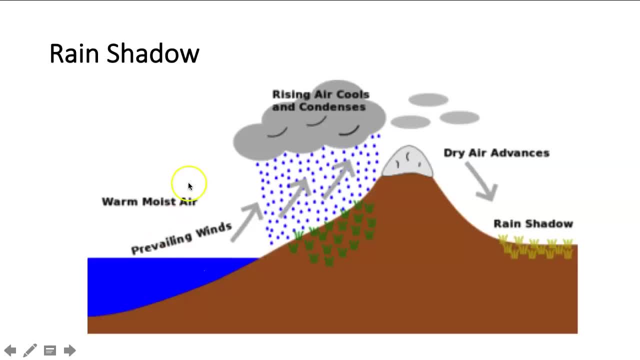 So, for example, the Andes in South America, that air is going to head in towards the mountains, so like my arrow there. but it kind of gets stuck in a way on those mountains and what that does is it forces a lot of that air up. Well, just. 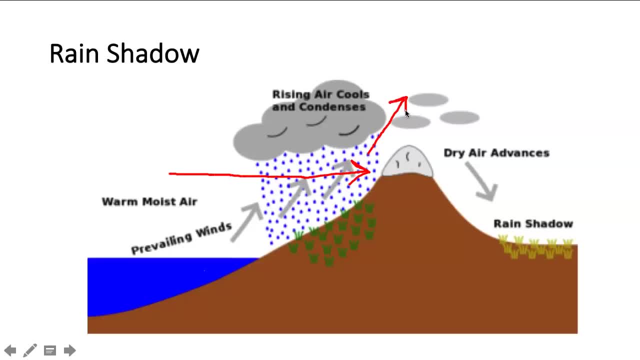 like with Hadley cells, where a lot of the moisture gets released as the air rises because it's cooling and condensing, you're gonna see all of that rain drop On the windward side of the mountain Well after we have the windward side of. 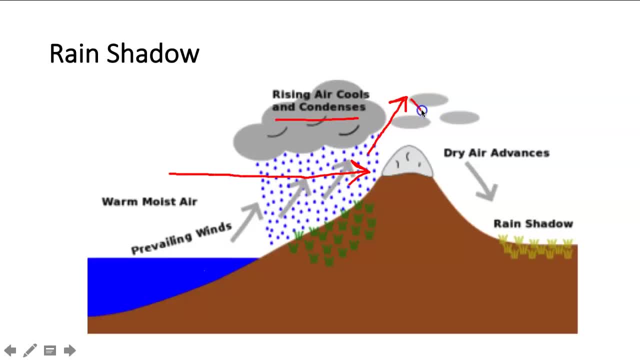 the mountain getting soaked in all that rain. all that cold dry air is going to make it to the leeward side of the mountain. So very much again like that Hadley cell circulation where the cool dry air kind of wraps around to the 30. 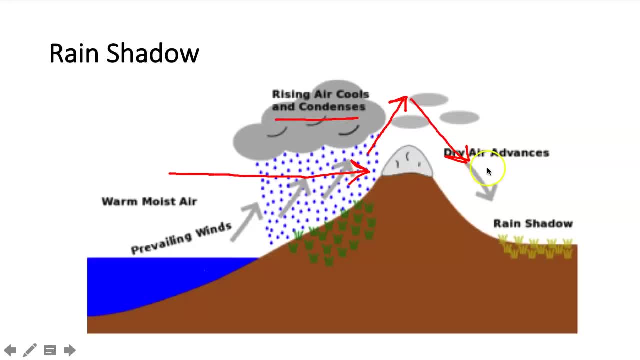 degree mark. in this case, it's just going over a mountain. instead, You can see that cool, dry air coming around the other side and as it approaches the area where you're going to see your desert, it is going to be very dry. It's going to start to warm up, approaching the surface of the earth. 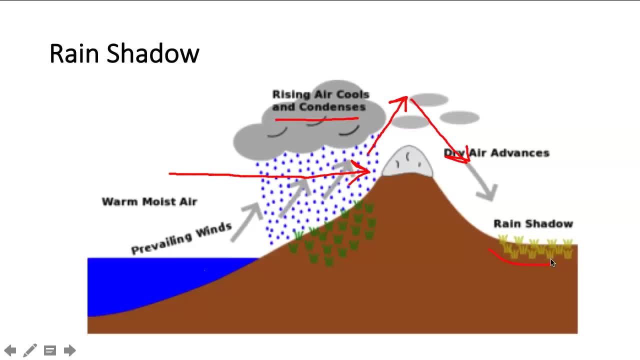 again and it is going to create those hot, dry desert areas on the other side of the mountains. So again, we see these with the Andes in South America. We also see them with the deserts that are found where Nevada is as well, due to the 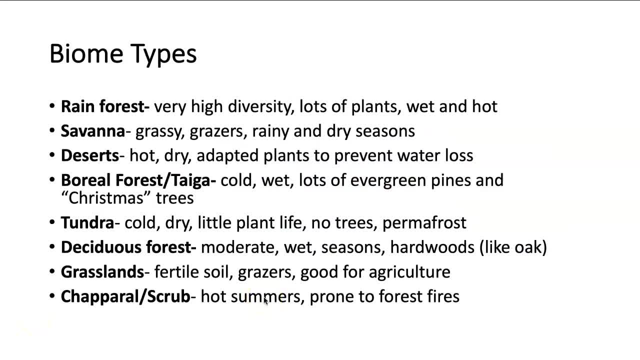 mountains in California. Alright, here's a real quick overview of your biome types that you should be familiar with. We all pretty much know that rainforests have lots of plants and that they're also very wet and very hot and located near the equator Basically. 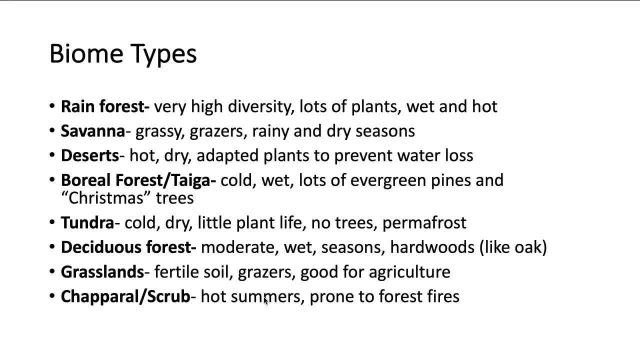 your biome pictures that you guys did in class, where you colored everything in to kind of get a general gist of where they're located around the earth. you should be familiar with that as well. We should know that savannas are going to be grassy. There's lots of grazers, but one of their key facts is that they have 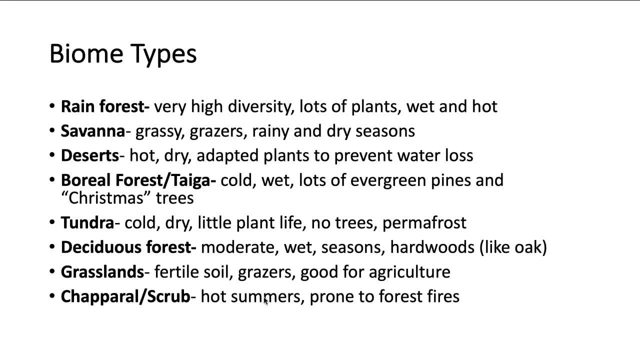 rainy and dry seasons, so they can be prone to fires as well. Deserts, hot, dry, and then also know that the plants are especially adapted to avoid water loss. Just think cacti, Boreal forests and taiga, or even coniferous forests. all of those are interchangeable. They are going to be very 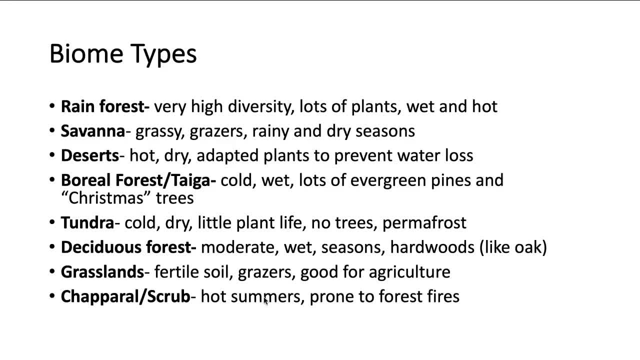 cold, wet, usually located right below tundras. So think like Canada or Russia. Lots of evergreen pines and what I just consider, Christmas trees. Just think about, when you go buy a live Christmas tree, what they look like. That's the kind. 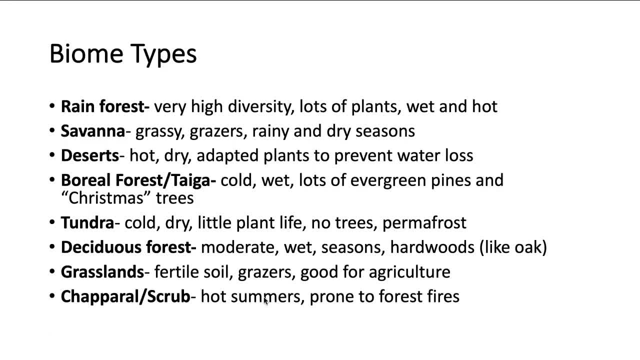 of trees you find in those areas. Tundras are found north of that. They're going to be near the Arctic Circle. So very, very, very northern Canada, Very, very cold, very dry, and you should know that permafrost, that frozen ground. 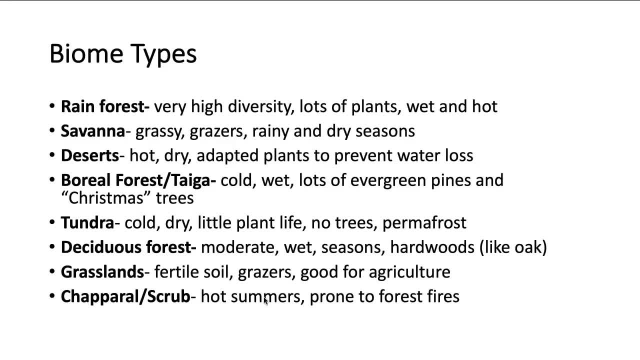 prevents tree growth because the roots are not able to penetrate into it. Deciduous forests- These are going to be our hardwood forests that we find in the eastern United States. Usually these areas are noted because they have four seasons. You're going to see again really warm summers. You're going to see cold. 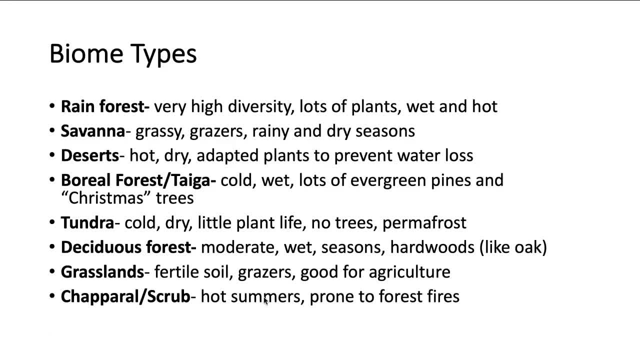 snowy winters and then your more moderate fall and spring Grasslands, the central part of the US or the Midwest. Good for agriculture, good fertile soil, Lots of grass, lots of grazers- in those areas as well, Kind of similar to Savannah, but not so much the rainy and dry seasons. And then 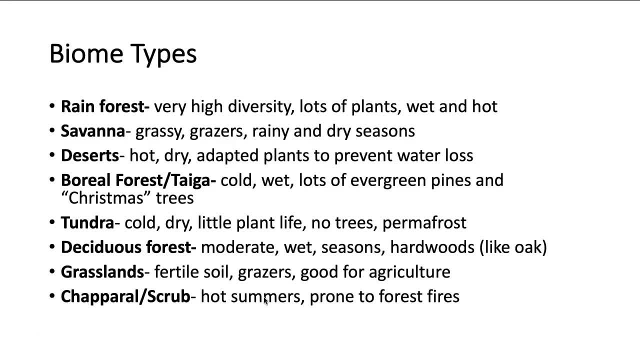 chaparral or scrub areas are going to have pretty hot summers and one of their main characteristics is they are prone to forest type fires in those areas. So when we see some of our California wildfires, a lot of those are due to that area not only being very hot and experiencing drought, but that chaparral. 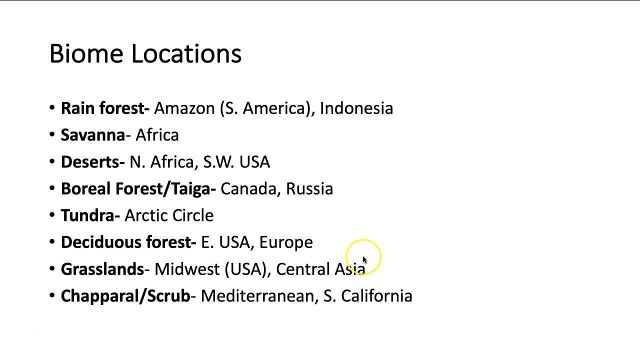 area also is common for fires as well. Okay, you might want to pause in just a second and review this list of common locations that we see, or well-known locations that we see these biomes in, because you will sometimes be asked to identify them on a map for the AP exam. 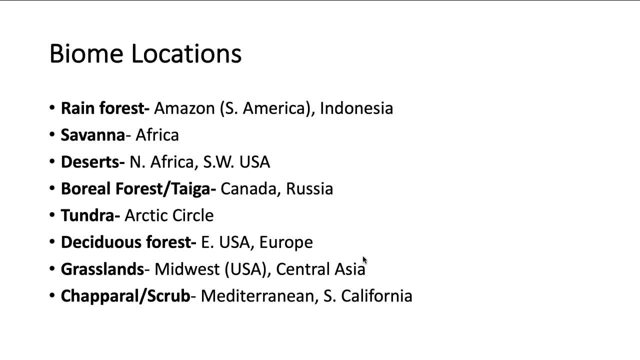 For me. I ask you a question about one of these, and you're going to need to be able to identify where it is. So if you paid attention to the map project that we did in class and saw, for example, that tundras are really far north, taigas are, 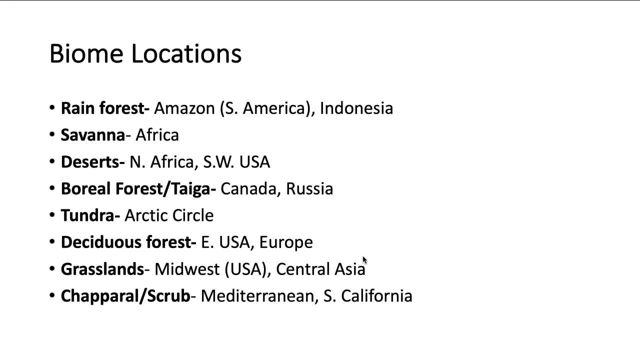 located right below. it tends to be in Canada and Russia that we see deserts again, just north and south of the rainforest at the Equator. you should be in pretty good shape, So hopefully your geography classes that you guys have had will come in handy here So you may want to pause, take a. 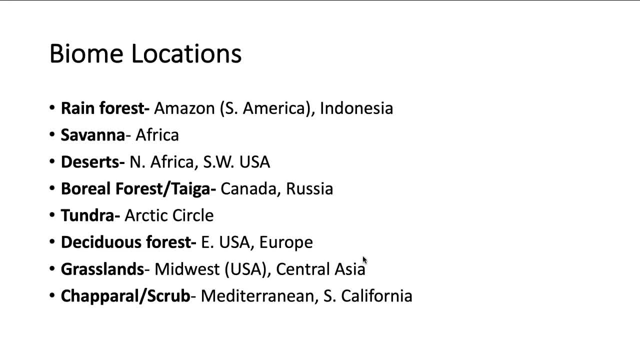 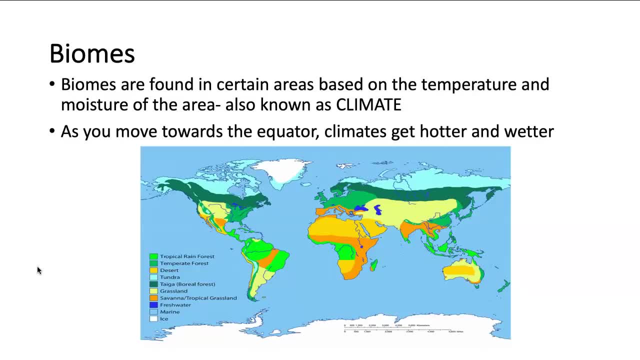 look over this and review it and then we'll move on to the next slide. All right, last big thing. I really want you to make sure you know, with your biomes You can review the map that I've got posted down there as far as where. 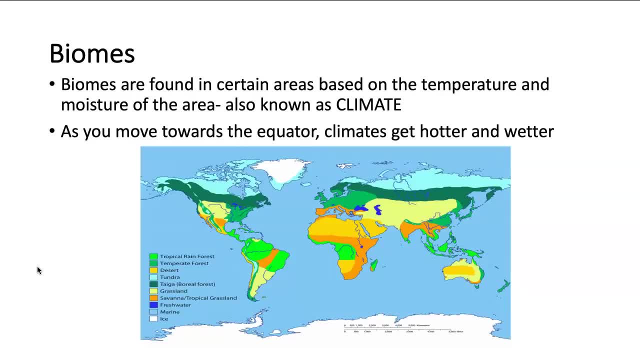 these biomes are located. In addition to that last slide that had the trees listed for you. but you should also know that climate is what determines where biomes are located. So if you have a very hot, very wet area, you are not. 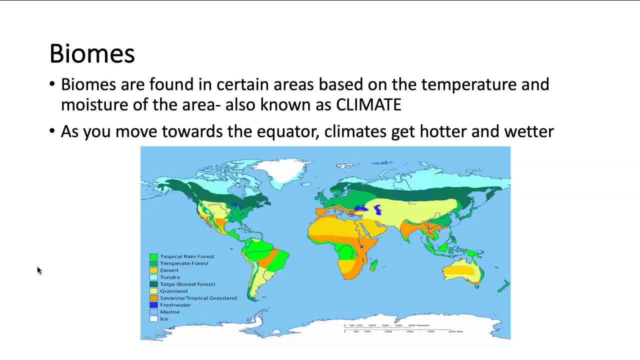 going to find a desert there. The deserts are hot and dry, So temperature and moisture of an area is really going to determine what kind of plant life, what kind of animals- whether or not there's rain, snow etc- is going to be there. And 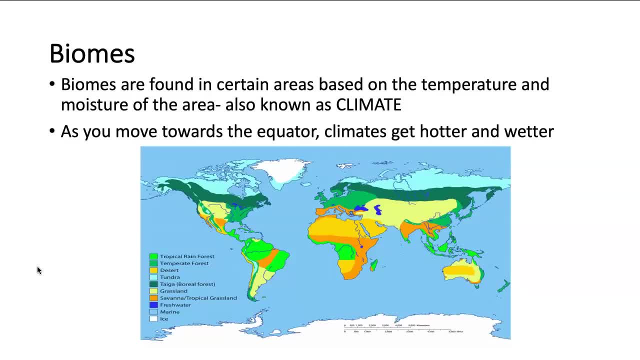 then also remember, as you move from the north or south pole toward the Equator, you're getting hotter and you're getting wetter, So you're going to have higher rainfall, higher temperatures on average. We do know that there are some exceptions, based on like how Hadley cell circulation works and whatnot, But in 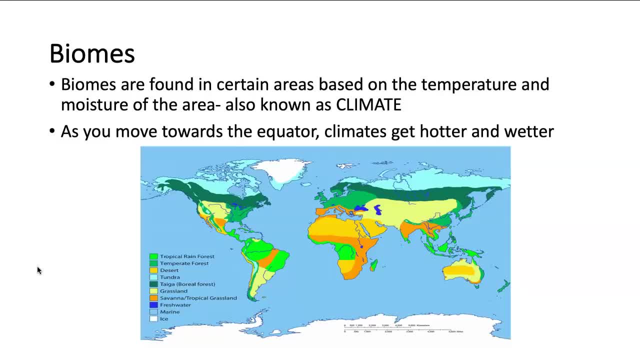 general, as you move towards the Equator, you're getting hotter and wetter, Or, if you start at the Equator and move toward the north and south pole, that you are going to be getting cooler and drier All right on to our aquatic biomes. So you 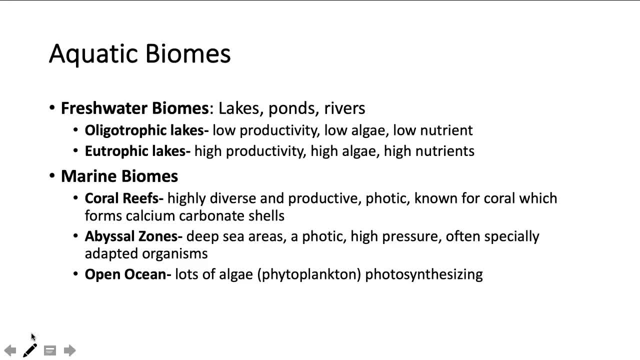 should be familiar with your freshwater and marine biomes, Kind of just the basics on these. You guys know what freshwater versus ocean is, But freshwater just know lakes, rivers and ponds are your big ones. You should know the difference between oligotrophic and eutrophic lakes, If you can remember. 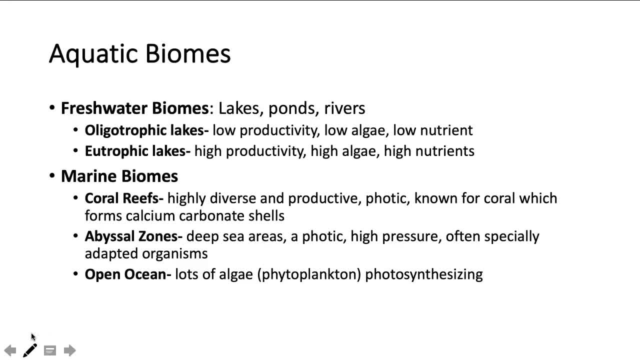 eutrophication, which meant a lot of algae growth due to nutrients. that's kind of what you get with eutrophic lakes as well. They're super highly productive because there's lots of algae and lots of nutrients there for the algae to grow. 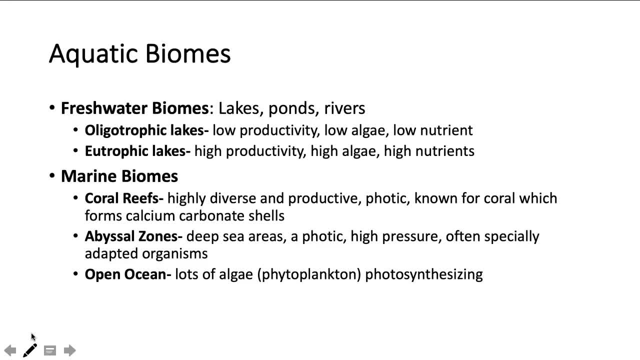 And then oligotrophic lakes are going to be your lower productivity. low algae, low nutrients. They're really clear, really pretty. You're going to find them in mountain ranges, for example. You're just not going to see the same amount of algae. 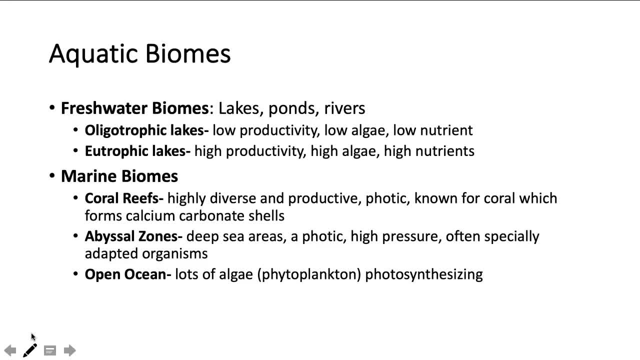 growth that you see in eutrophic lakes. So just think eutrophic lake eutrophication. both have to do with lots of algae, Marine biomes. you should definitely know coral reefs and definitely know abyssal zones. Coral reefs are super diverse, I think. lots of fish, lots. 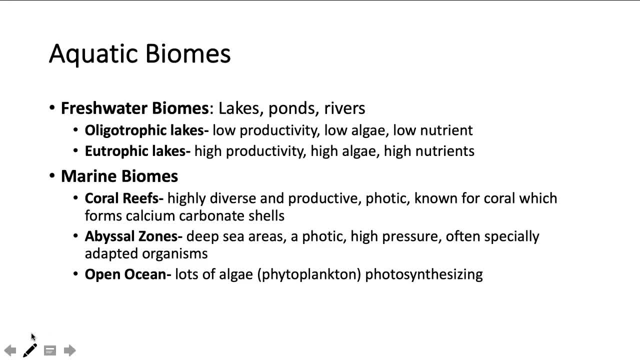 of different types of corals, lots of light, so they're in a photic zone And they're known for coral, which coral is made up of a calcium carbonate shell. That's kind of one of their defining characteristics for that, That ocean zone, Abyssal zones- think about our tubeworm assignment we did in class. They're. 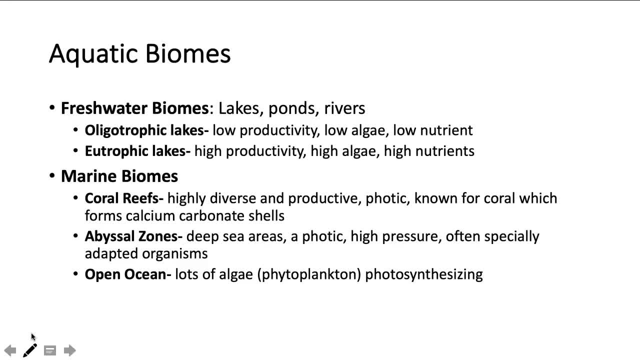 going to be super deep sea areas, super high pressure, absolutely no light. So they are considered aphotic And sorry, aphotic should be all smushed together in that word there: High pressure, and then also specially adapted organisms like the tubeworms we talked about. 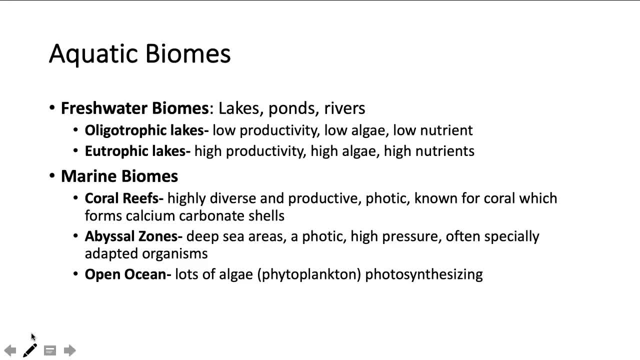 in class. So they might be doing chemosynthesis instead of photosynthesis, since there's no light, And then also know that the open ocean is full of lots of algae, which is also known as phytoplankton. So there's plenty of photosynthesizing going on. 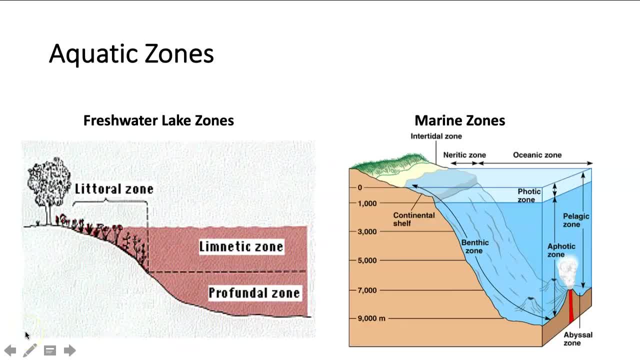 Okay, now for our freshwater and marine zones that you should be familiar with. You're definitely going to want to know your littoral and limnetic zones, So your littoral zone is going to be found right up here, near the coastline of any freshwater lake area or even near a river. 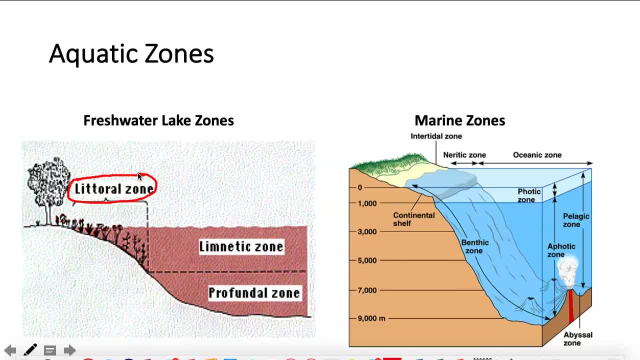 lake edge where you're going to have plenty of plant life growing in it. There's plenty of sunlight there, So think of it a little bit like the coral reef part of a lake. Limnetic is going to be more your open area, And then you should also know that benthic is going. 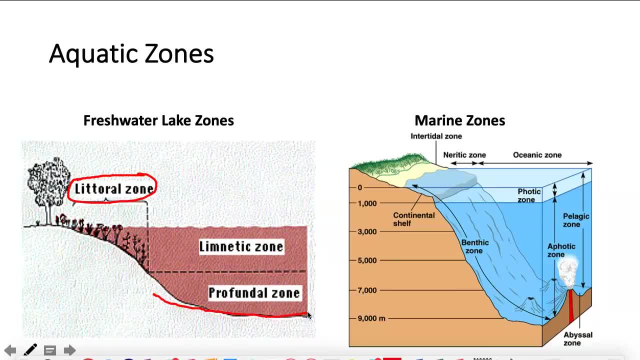 to be located at the lake floor. So I just drew that red line down there. But littoral and limnetic are the two ones in particular to freshwater lakes, you should know. And littoral, near the edge of the lake, plenty of plants. Limnetic is kind of the open part of the lake. 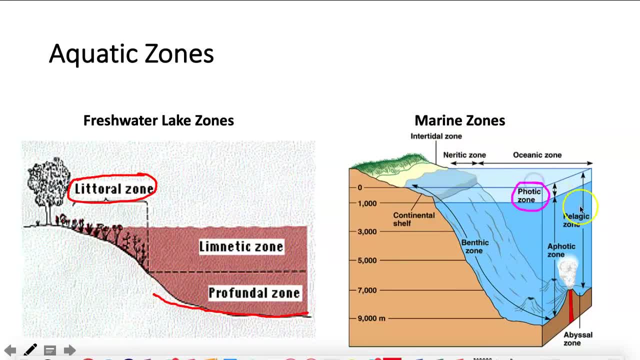 So if you have a lot of water, you should definitely know that benthic. So that's going to be your middle zone. And then you should also know your subtropical zone, which is your inner tidal zone. So you should know that the inner tidal zone is going to be your upper. 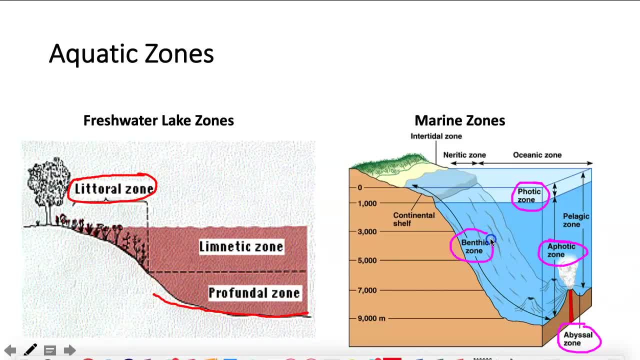 tidal zone. So that's going to be the inner tidal zone. And then you should definitely know your photic and your aphotic, So light and no light zones. You should know the term abyssal zone So you see down where our hot vents are, like we learned about with tubeworms. 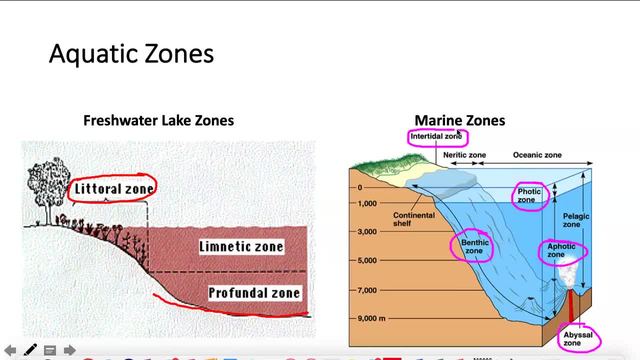 in class Benthic again, is that sea floor or lake floor? if you're talking about lakes, Those are going to be your big ones parts of the time. it's kind of inconsistent for them, So they're specially adapted to not. 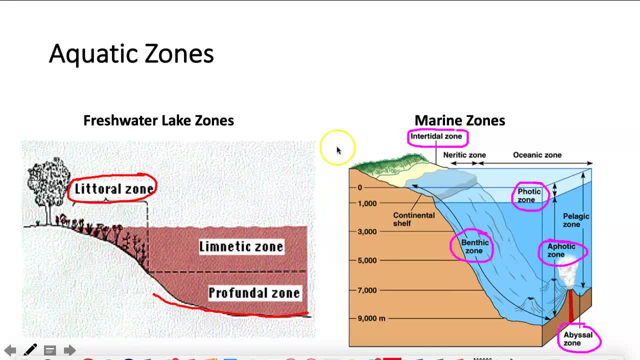 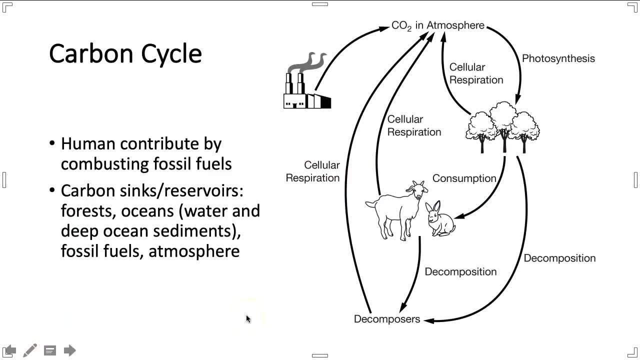 be solely underwater type organisms. So those will be your big ones for your different types of zones. All right. now on to your biogeochemical cycles. Big one here is going to be carbon cycles. So what we need to know with that, there's a picture over on the right that you will see. 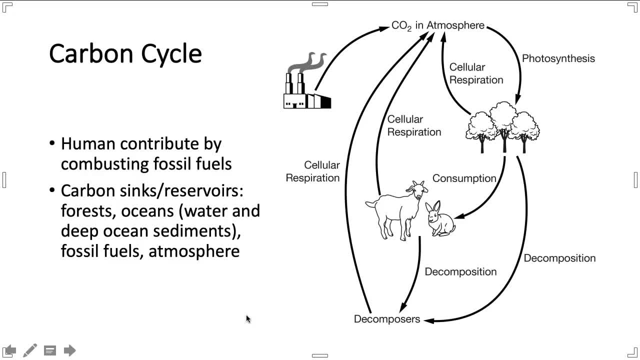 on your test and you'll have various questions attached to that. So I thought I'd go ahead and give you the little preview of this mini version of the carbon cycle. You guys know it's way more complicated than that picture, So you should know that humans contribute by combusting fossil fuels. 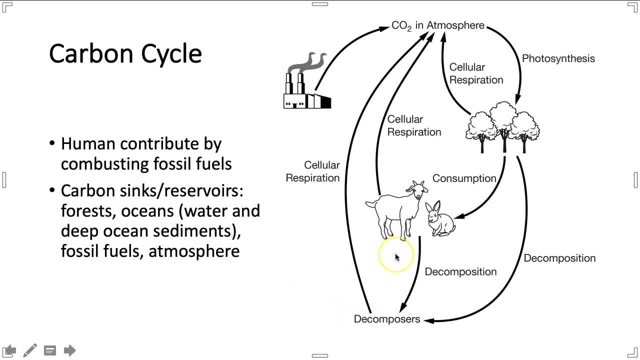 and that we also have carbon sinks and reservoirs, including things like forests, So trees, for example, because they live so long. Oceans, so not only the open water, but also deep ocean sediments, fossil fuels, the atmosphere, rocks and soil- the things that we went over with your. 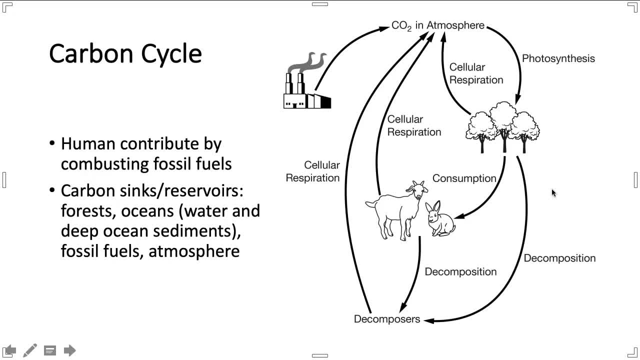 carbon cycle game in class should help you with those. Now other things with carbon cycle. you should know You can see again that human controversy- sorry contribution over here with industry That's going to be a big part. You should know your little mini cycle that we talked about with cellular respiration releasing carbon dioxide. 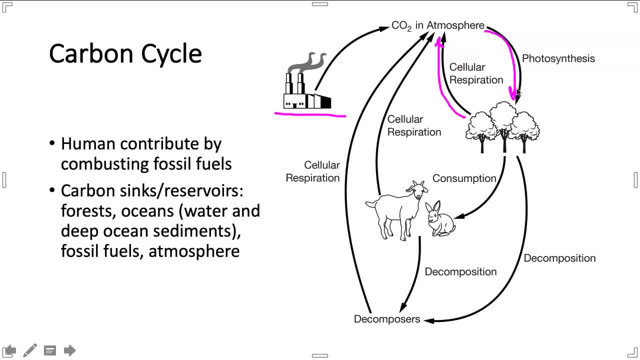 photosynthesis, bringing carbon dioxide back into plants to help convert it so that organisms can use it. And that's the plant part of it. right there You can see cellular respiration coming up from animals over here as well. Decomposition is going to be another big part of it. Decomposition. 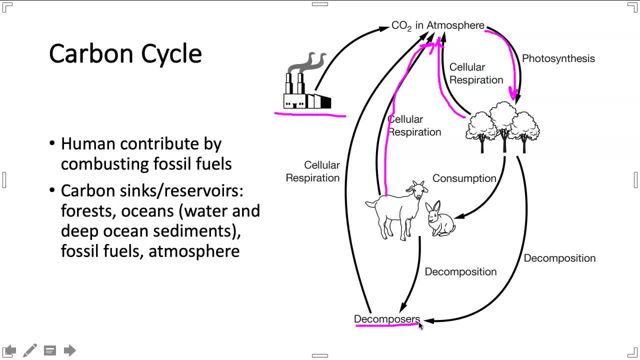 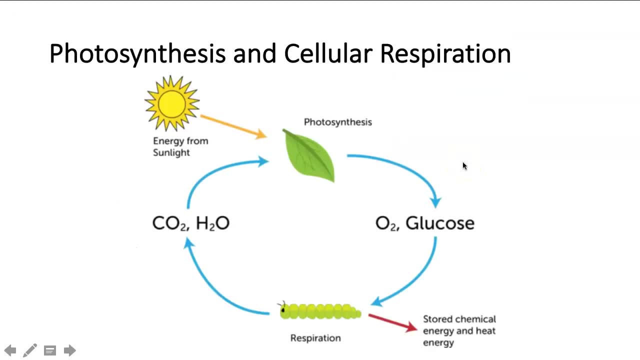 can eventually lead to fossil fuel formation over millions and millions of years. And those are going to be all your big key components right there Again, that human contribution through combustion, photosynthesis, cellular respiration. those are going to be the big things that you need to know. All right, so just to touch on. 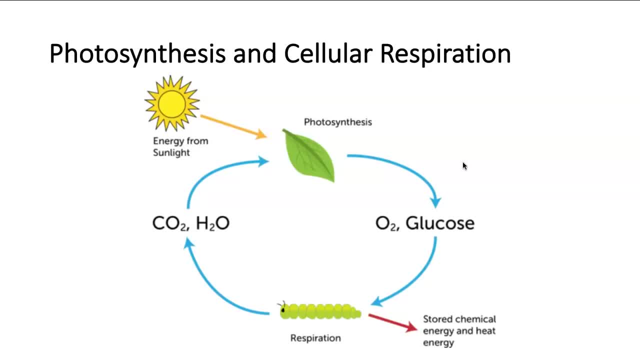 photosynthesis and respiration a little bit more. here is that cycle in and of itself. You can see, with photosynthesis you're producing oxygen and glucose, which is a carbon compound from carbon, carbon dioxide and water being taken in. So glucose, remember, is C6.. There's your carbon. 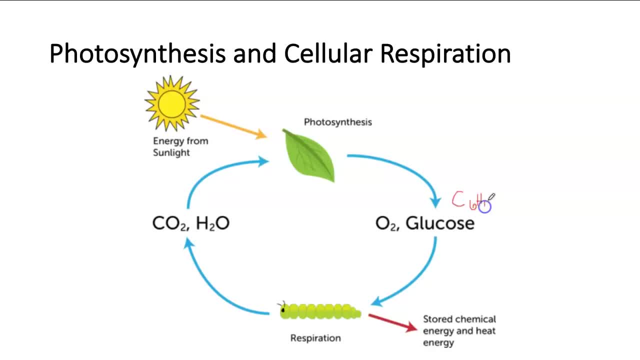 part H12O6.. You should be familiar with its actual formula. So that's where that carbon dioxide going in is being converted into another carbon compound And then animals- insects, for example- are going to take in that glucose and they're going. 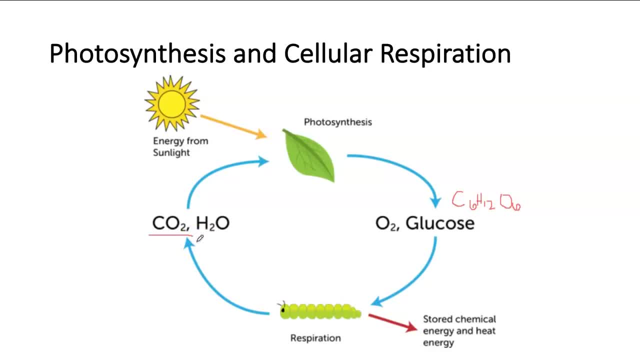 to respire and breathe out the CO2.. So that's its own little mini cycle within the carbon cycle. You should be familiar with it that photosynthesis pulls carbon dioxide out of the atmosphere, Respiration adds it to the atmosphere And then respiration is also going to take in. 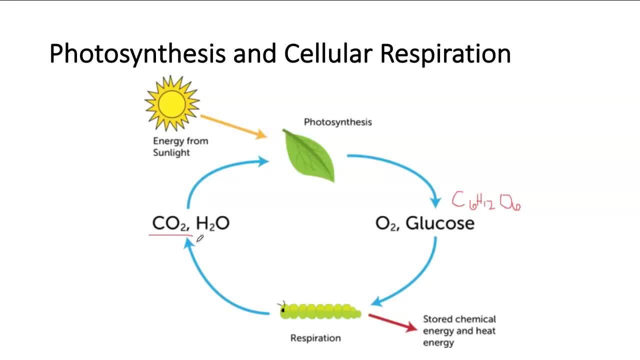 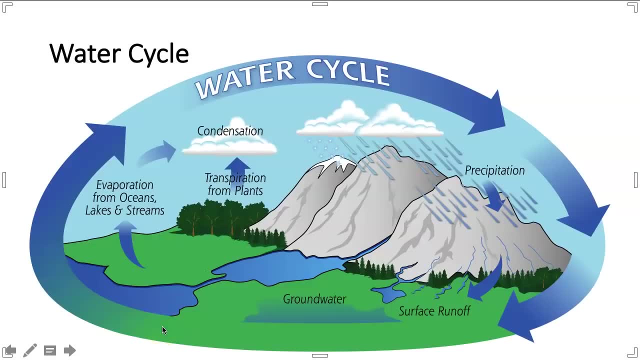 glucose its carbon compound as well, but that's not an atmospheric form of carbon, It's just a sugar compound. You should also be familiar with the major steps of the water cycle. I gave you a little picture here that shows a few of the key things. So you should know that evaporation is water. 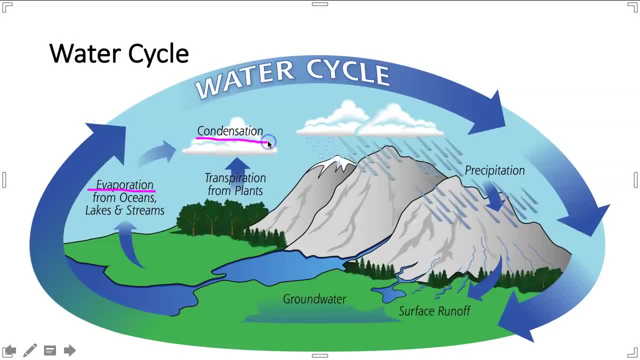 going from liquid to gaseous form. Water can condense and become clouds or water vapor That can rain, So that's precipitation, And notice that shows snow and rain. Snow is actually a form of precipitation. Precipitation can lead to runoff And that runoff can actually become part of 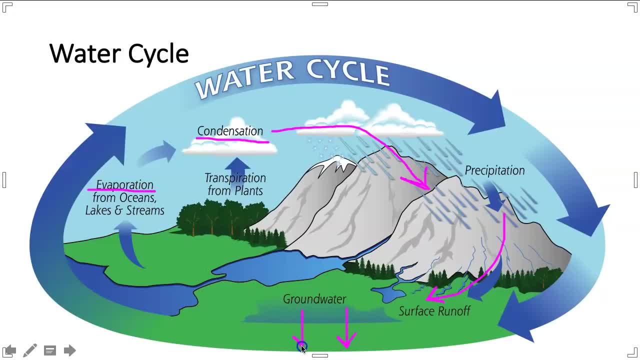 groundwater through percolation- which is not on here but it is on your notes- And then we can have that water also go back into surface water, which can then start everything over again with evaporation, transpiration, which is evaporation off of plants, and everything just continues to cycle. So just be familiar with 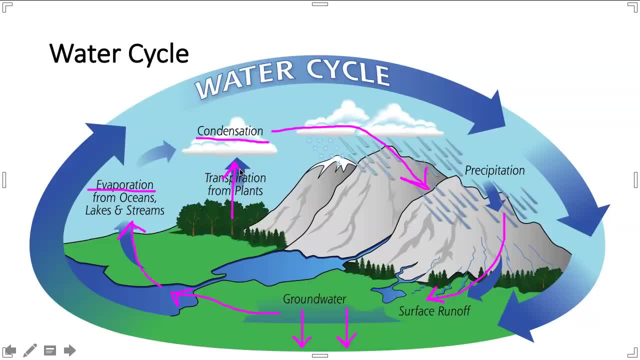 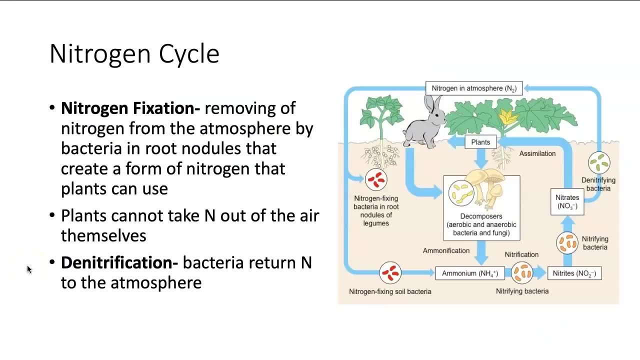 those main parts of the water cycle. You will have a picture and you will have to be able to identify what they are. Key parts of the nitrogen cycle that you'll need to be familiar with are listed on this slide, And then you can also. 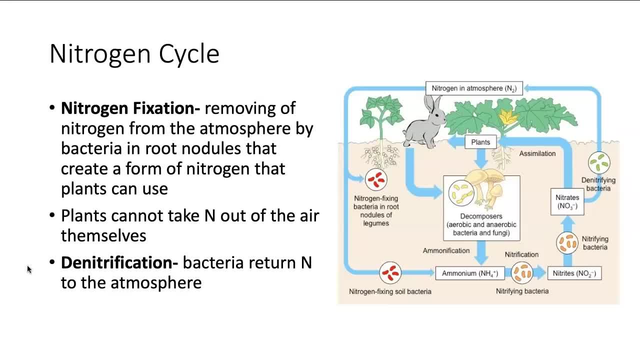 view the diagram from your notes that we did with Bellwork, where I had you guys labeling some compounds. Definitely no nitrogen fixation, which is where bacteria is pulling nitrogen out of the atmosphere and it is using its roots, or sorry, the bacteria is located on the roots of the plants. 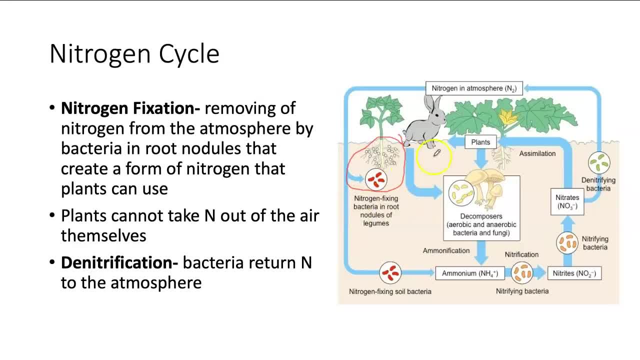 So plants are using the bacteria located on their roots to undergo nitrogen fixation, which is going to help pull that nitrogen from the atmosphere. That's going to create a plant friendly form of nitrogen that can be used. So you can see that the bacteria is not able to take nitrogen just right out of the atmosphere themselves. 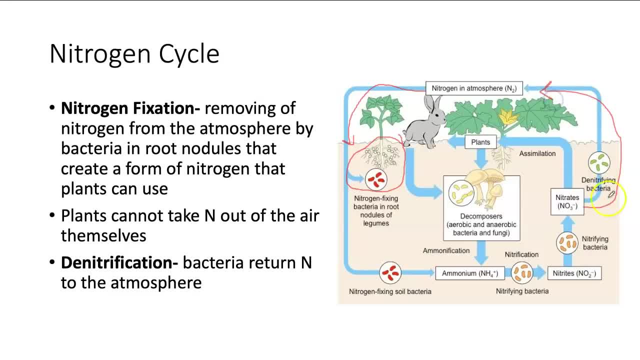 You should also be familiar with denitrification, which is kind of the opposite, where nitrogen is being released by bacteria back into the atmosphere. So those are going to be your big ones. You can see there's also what we talked about in class with. 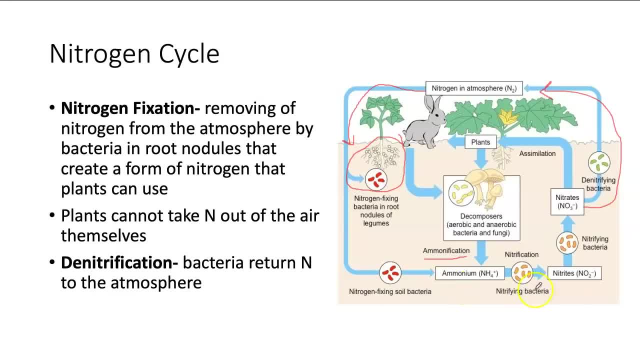 ammonification, where we have ammonia being converted by bacteria. Notice, a lot of bacteria is involved in the nitrogen cycle. That's going to be one of the key components is just the bacterial involvement. So, again, nitrogen fixation, Bacteria being pulled or bacteria pulling nitrogen from the atmosphere, while they're attached to the roots of plants to make it accessible to the plants. 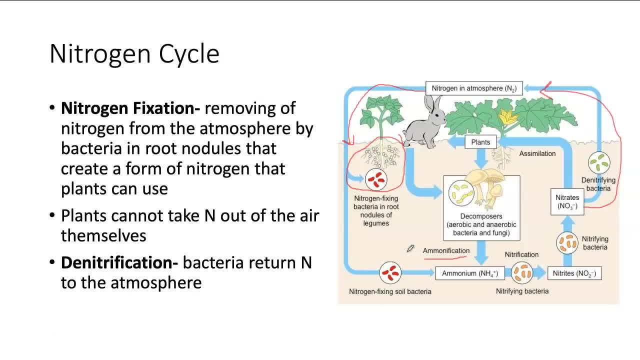 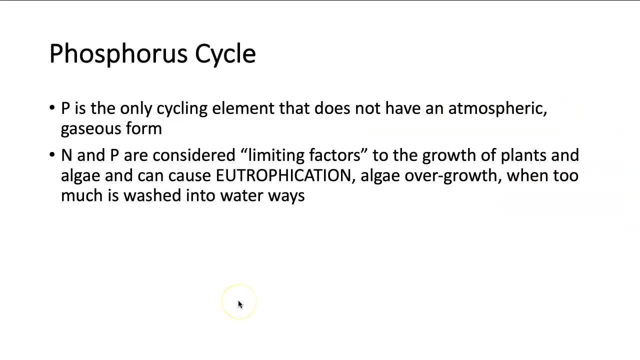 That's actually a form of symbiosis and denitrification- the release of nitrogen into the atmosphere by those similar kind of bacteria as well. For phosphorus cycle, the main thing you need to make sure you remember is that phosphorus does not have an atmospheric or gaseous form. 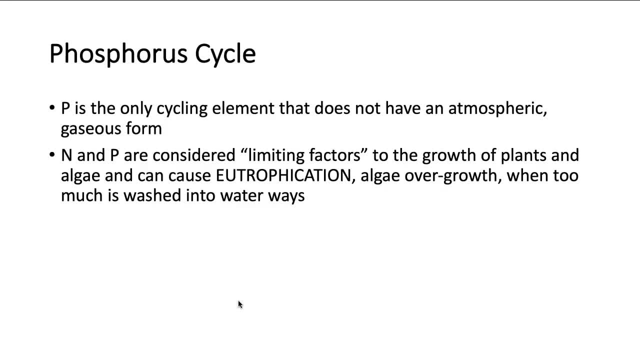 So we see it cycling through plants and animals. It's organic forms. We see it also cycling through rocks. The main way it makes it into the environment from the rocks is through weathering, So part of the phosphorus kind of gets washed away by different environmental factors. 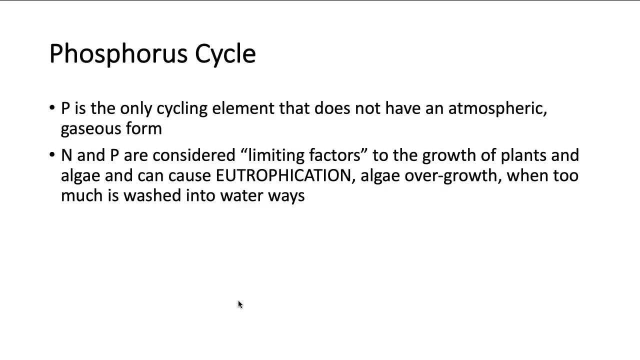 You should also know that nitrogen and phosphorus are considered limiting factors for the growth of plants and algae, So this is why we often use them in fertilizers, which we'll talk about with water pollution later in the year. But for now, what you should know is that too much of those fertilizers can cause eutrophication. 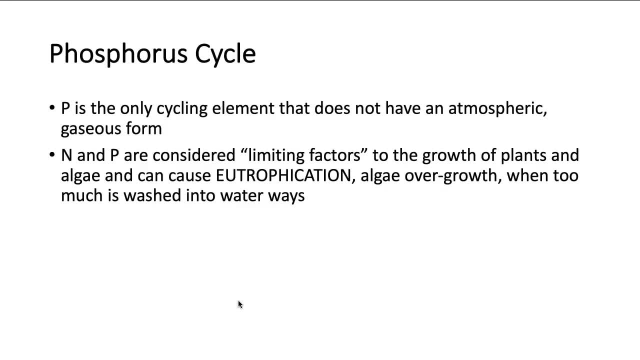 Or algae overgrowth, when too much ends up washed into waterways. And then we know that algae can also end up dying, eating up oxygen as it's decomposing, and that can end up causing hypoxia or a lack of oxygen in the water. 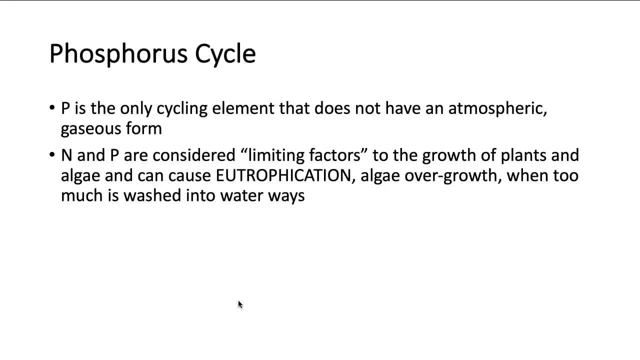 And that, ultimately, is why eutrophication is such a problem for other organisms within aquatic biomes. All right, so those are all the key components of the Unit 1A test that you need to make sure you are aware of. So watch this video as many times as you need.